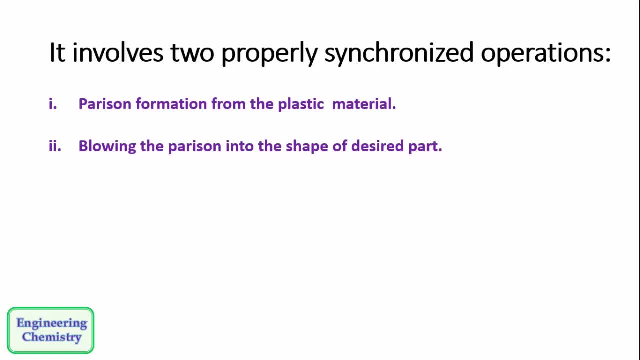 And second is blowing the parison into the shape of desired particles. There are two types of techniques which are used in the blow molding. The first is extrusion blow molding, which is characterized by scrap production, And the second is injection blow molding, which is versatile, scrap free and is accepted by processors. 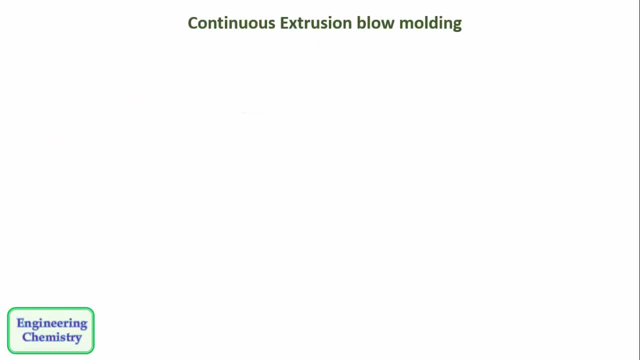 First we will see extrusion blow molding. There are two types of extrusion blow molding. First is continuous and second is intermittent. First we will see continuous extrusion blow molding. In continuous process, a continuous parison is formed at a rate which is synchronized with the rates of part blowing, cooling and removal. 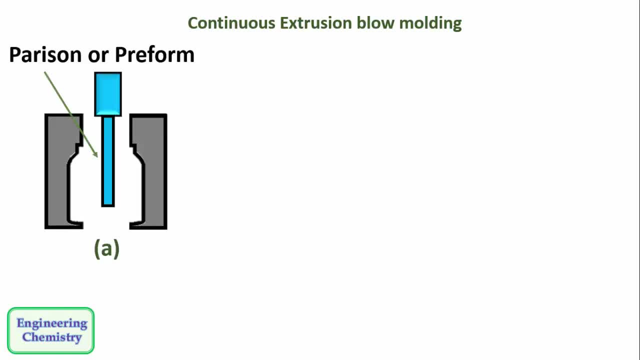 As you can see in the diagram, the parison is first placed between the halves of the mold. In the second step, the mold closes around the parison. In the third step, the parison still blows. In the fourth step, the parison is pinched off and inflated by an airblast that forces its wall against the inside contours of the cooled mold. 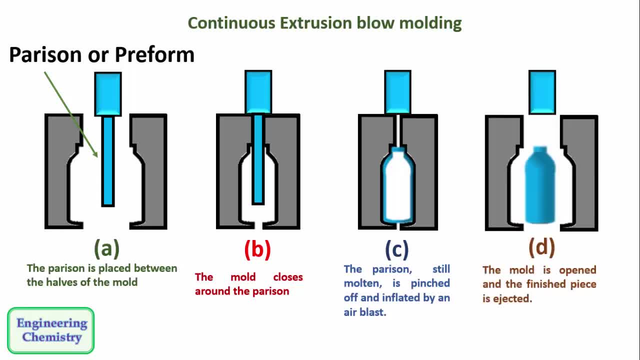 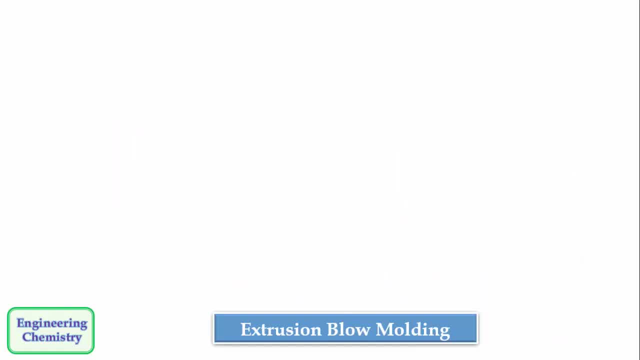 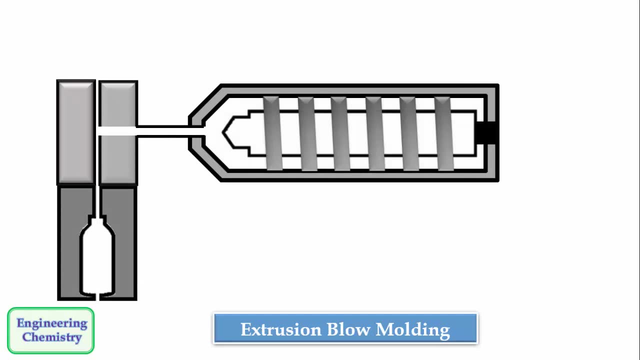 In the fourth step, when the piece has cooled enough to have become solid, the mold is opened and the finished product is ejected. Let us see now intermittent extrusion blow molding. The equipment is same as that of injection molding, as we have seen in the earlier video. 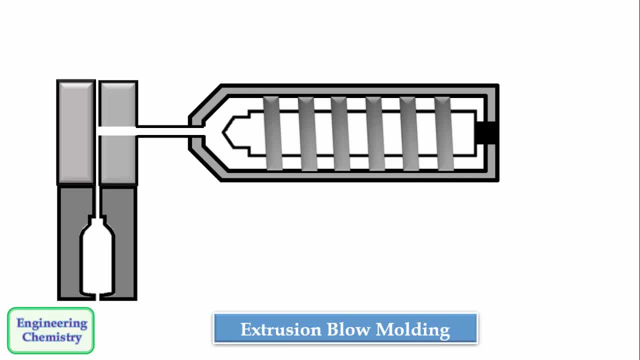 It consists of a machine with the respective mold parts. It has a hooper at the top and a motor aside. In extrusion blow molding, an extruder is used to plasticize the resin and form the parison. For this, we will take all the ingredients which are required to manufacture the material into a hooper. 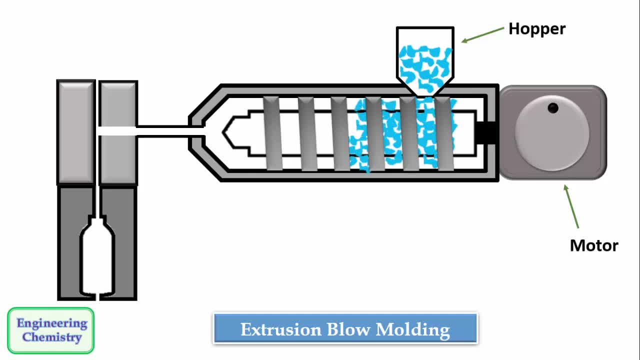 With the gravitational force it is taken inside the machine. When we start the machine, we will take the ingredients which are required to manufacture the material into a hooper. We will start the machine. we will start the machine. All the ingredients are pushed into the heater region. 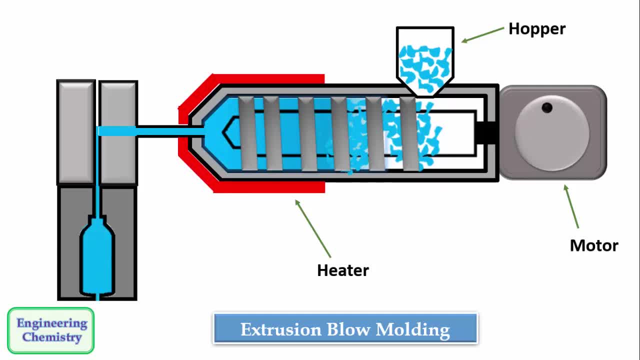 Parison from a molten thermoplastic resin is then entrapped between the two halves of the mold of a desired shape. Air, usually at about 100 psi, is blown into the soft parison. It is followed by curing process. The part is cooled and removed from the mold.